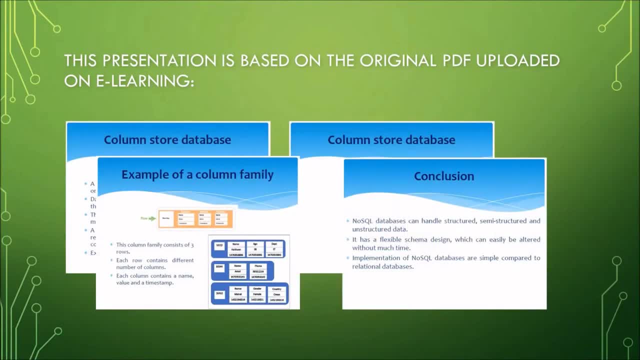 This video presentation is based on the original PDF uploaded on eLearning. Good day everyone. Again, I hope you're all safe and well. Welcome to part 5, the last part of this NoSQL video series. So let's get started. 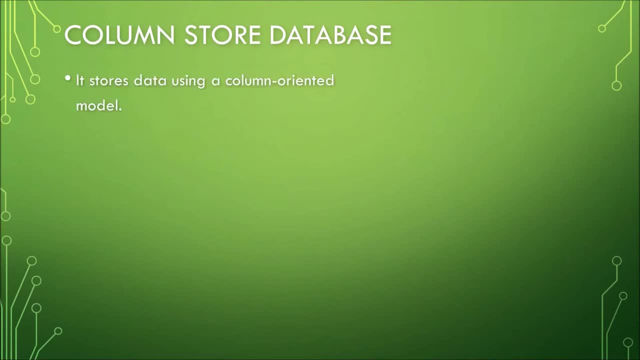 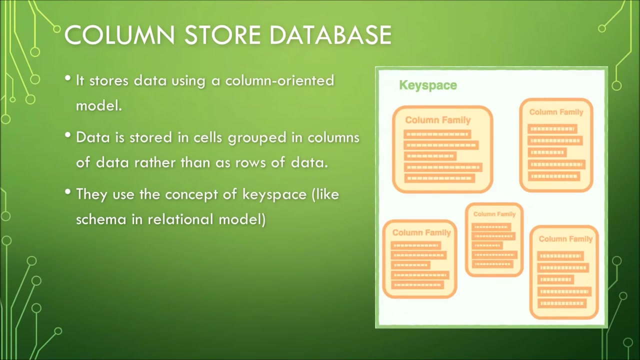 Now ColumnStore database stores data using column-oriented model. Now data is stored in cells grouped in columns of data rather than as rows of data. They use the concept of keyspace. It's kind of like a schema in a relational model. So in a relational model, schemas give us a view or structure of the entire. 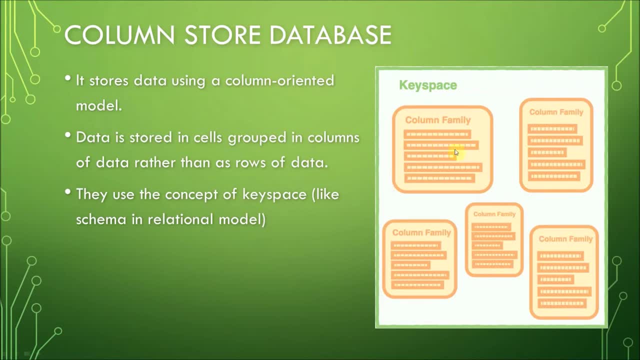 database In a ColumnStore database. a keyspace here. a keyspace will give us an idea of the entire structure of this ColumnStore database. So let's get started Now. a keyspace contains column families. So here are column families here in this. 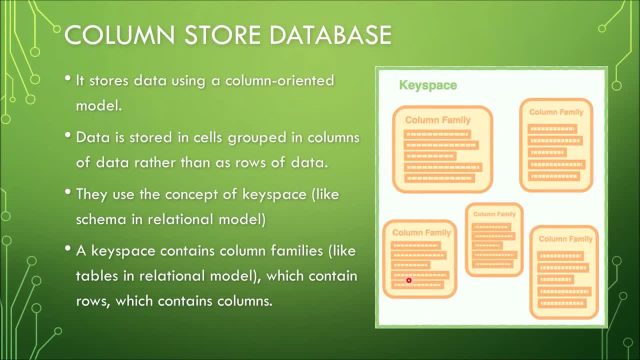 example, keyspace One, two, three, four, five column families. Now, column families here are kind of like tables in a relational model. Column families contain rows, So these are rows And within each row there are columns, as expressed in: 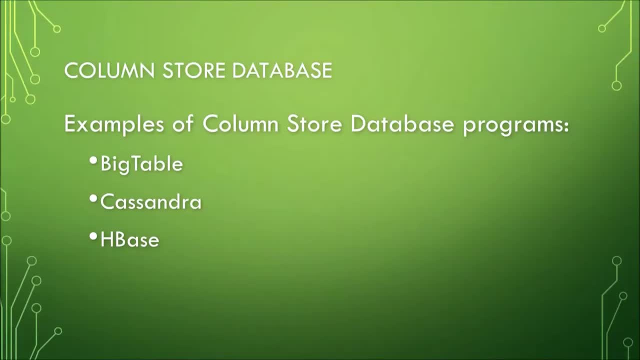 this example here Now. examples of ColumnStore database programs are Bigtable, Cassandra, HBase and there are a few other database programs that support ColumnStore databases. Now, column-based NoSQL databases are widely used to manage data warehouses, business intelligence, customer relationship management, or CRM, and library card catalogs. Now let's take a look at an example of a column family. Now, let's take a look at an example of a column family. Now. ColumnStore databases are widely used to manage data warehouses, business intelligence, customer relationship management, or CRM, and library card catalogs. 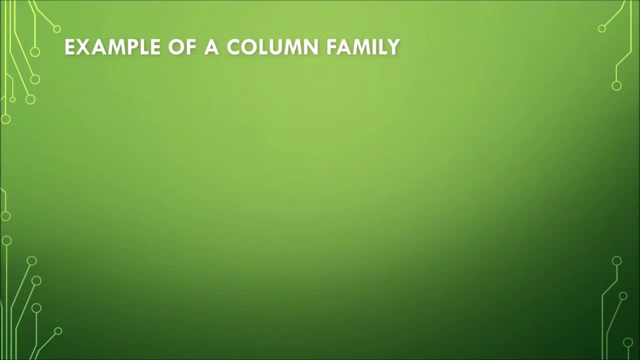 Now let's take a look at an example of a column family: Now ColumnStore. databases are widely used to manage data warehouses, business intelligence, customer relationship management or CRM and library card catalogs. Now let's take a look at an example of a column family Now: ColumnStudentscom. 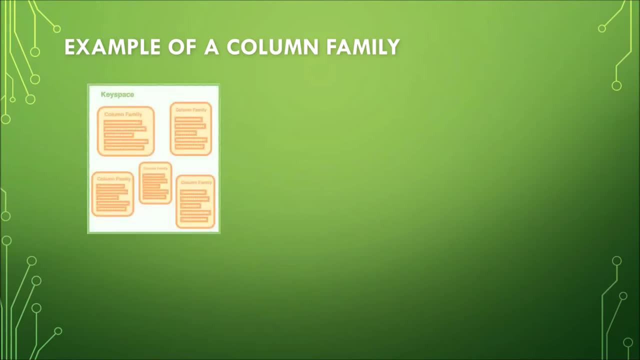 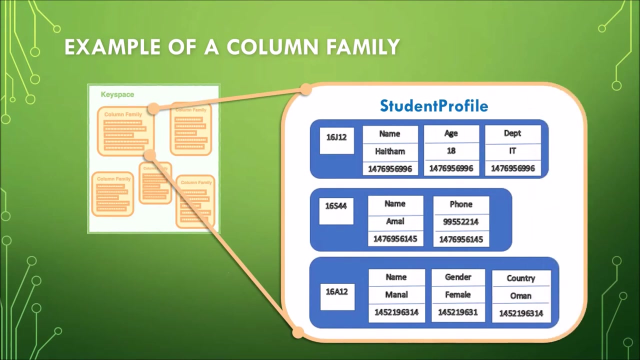 Now the structure of a column store database begins with a keyspace. right Again, the keyspace contains all the column families. Column families are like tables in a relational model. In this example we have a StudentProfile column family. This column family consists of three rows. 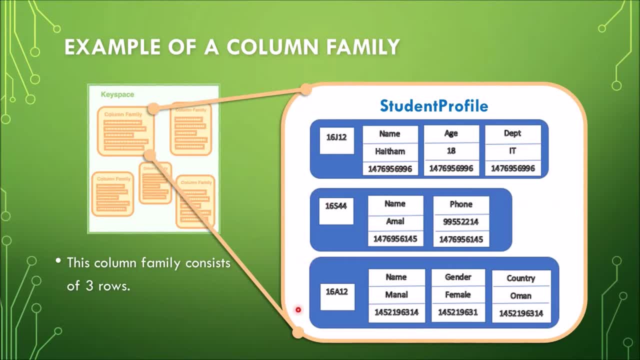 So this is the first one, This is the first row, This is the second row, the second one and the third row. as you may have noticed, each row contains different number of columns. in this first row, we have the column name, age and department. in this second row, we only have 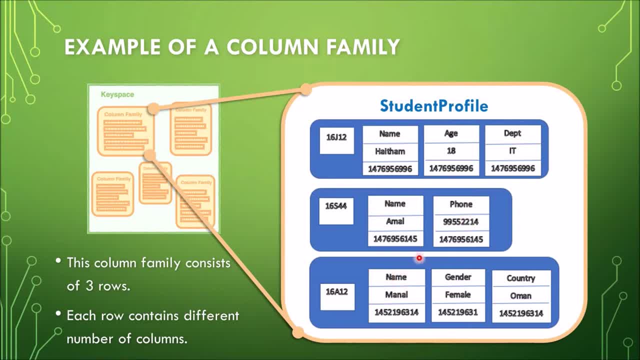 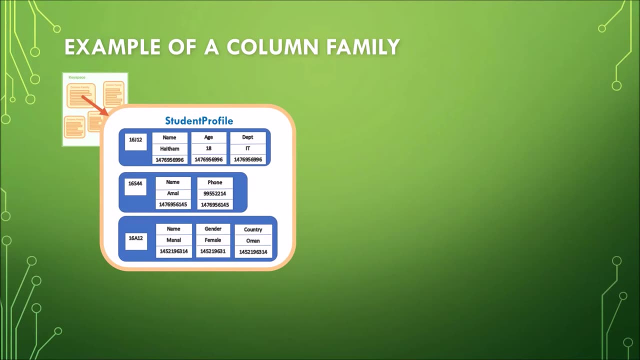 name and a phone, and on the third row we have a name, a gender and a country. so what this means is that the columns don't have to match the columns in other rows. they can have different column names and different data types. so let's take a further look at one of the rows of this student profile. 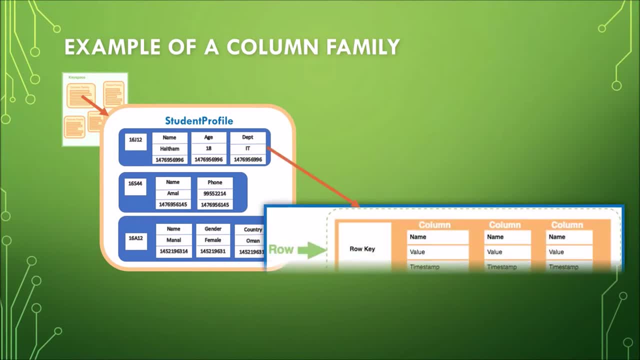 column family. as you can see in here for each row there are columns. so this row here there are three columns in this example. for now each column is contained to its pro and it doesn't span all rows like in a relational database. we don't do it like that. in relational database one column spans several records. 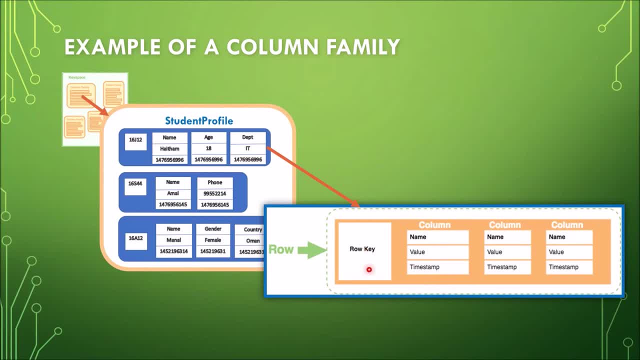 but in here a column is contained within a row. now each column contains a name value pair. as you can see, in here we have a name, a value, so there is a name value pair along with a stamp. note that this stamp in this example here uses unix epoch time for the timestamp. 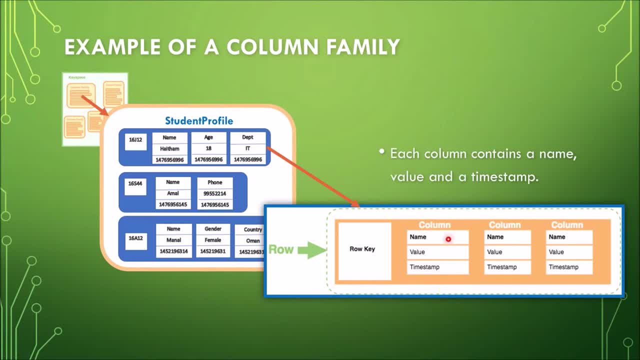 again. each column contains a name, a value and a timestamp. so here is again the breakdown of each element in the row. this is your row key. each row has a unique key which is a unique identifier for that row. it's likened to a primary key and then we have the columns. 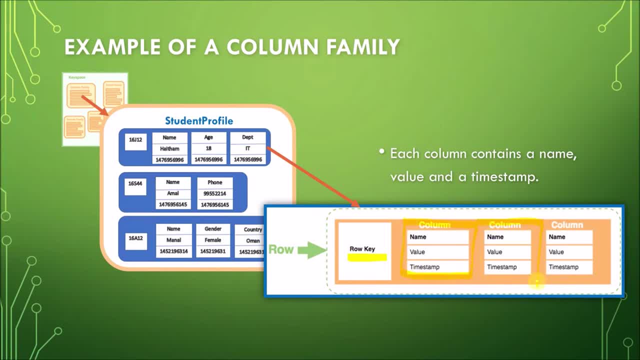 so this is one column, another column and another one. now each column contains a name, a value and a timestamp, and so it goes with the rest of the columns: name, value, timestamp. name value, timestamp. so this is the name, the name is the name of the name value pair and obviously the value is the.